wiped out the large crater. The moon's surface is also known as the largest crater in the world. The moon's surface is known as the largest crater in the world. It is also known as the largest crater in the world. It is supposedly the largest crater in the world. 3. The impact of the impact craters. The impact craters is a sign that the Earth is in a state of crisis. The impact craters are the most important ones. They are the ones that have the most impact on the planet. They are the ones that have the most impact on the planet, You might think. 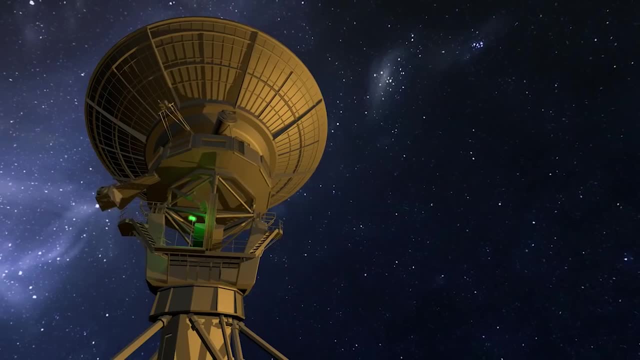 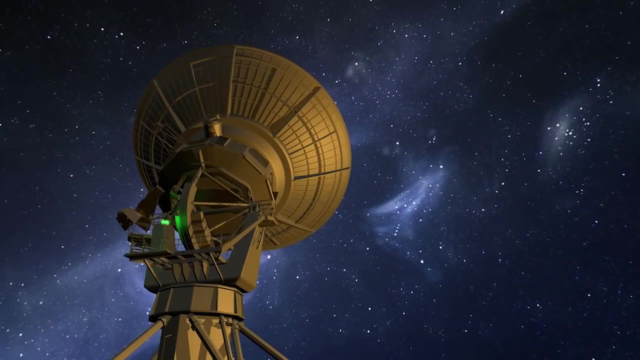 but why does that matter? Scientists like to use impact craters to help determine certain things about the surface, as well as indications of where to look for materials of asteroids or meteors that might have pelted the surface of certain moons or planets. 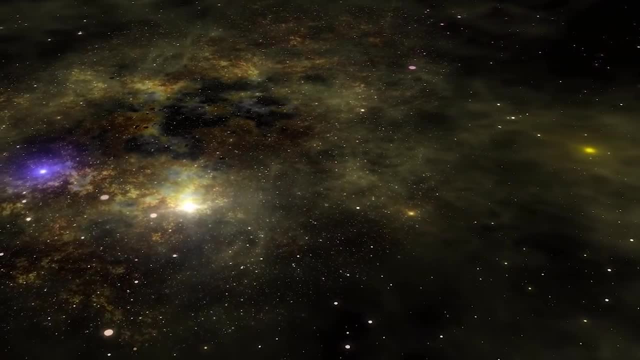 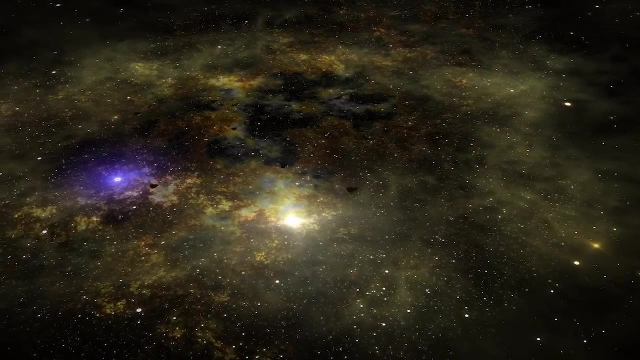 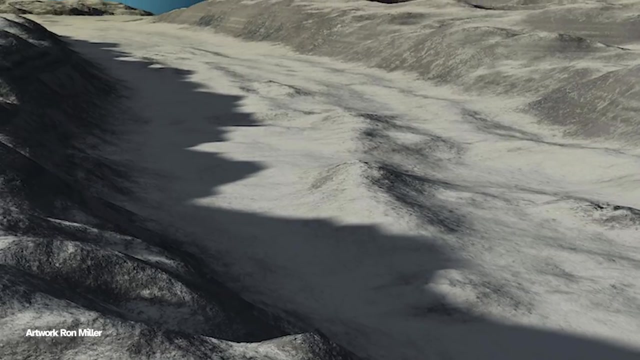 Because getting samples of them can help tell a timeline for various things, including the history of the planet. Ariel is also thought to have the most recent geologic activity of Uranus' larger moons. It is transected by grabenes, which are fault-bounded valleys. 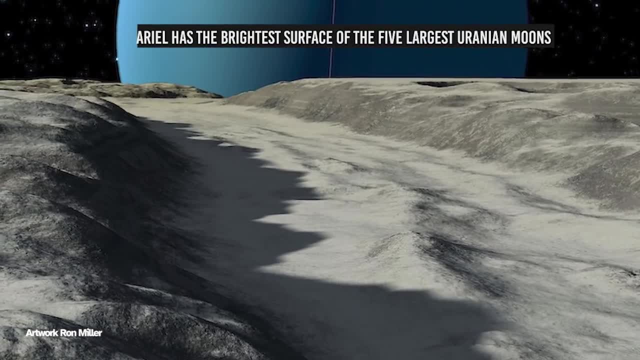 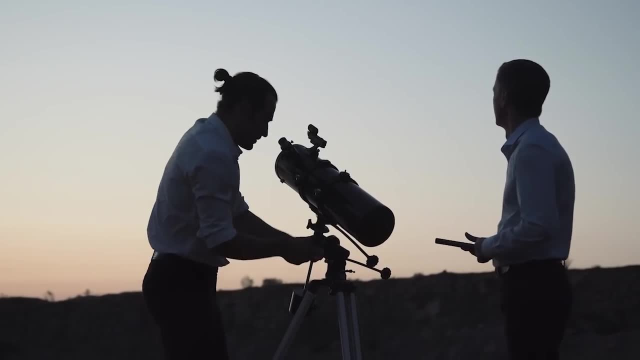 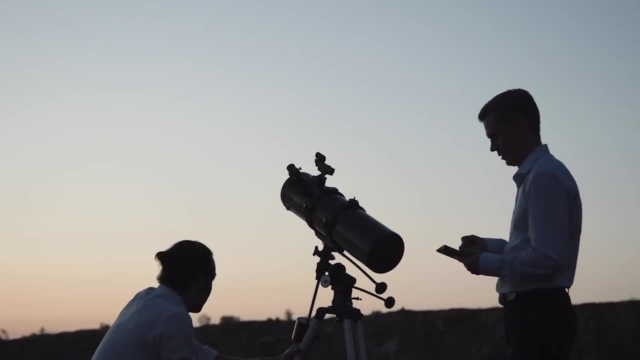 Ariel has the brightest surface of the five largest Uranian moons, but none of them reflect more than about a third of the sunlight that strikes them. This suggests that their surfaces have been darkened by a carbonaceous material. Ariel's brightness increases dramatically when it is in opposition, that is, when the observer is directly between it and the Sun. 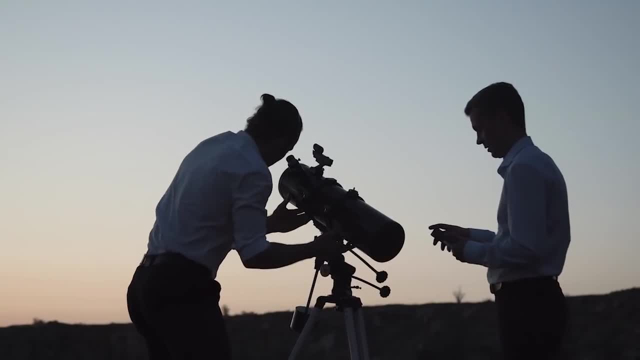 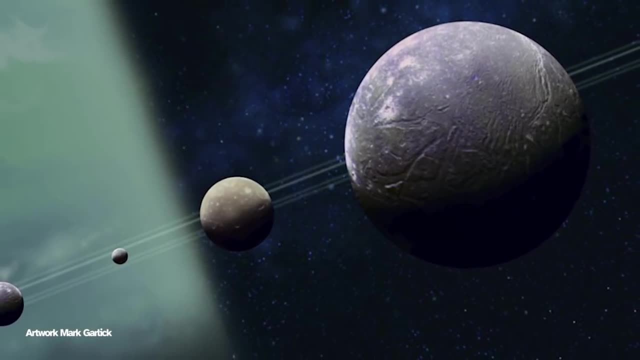 This indicates that its surface is porous, casting reflectivity, decreasing shadows when illuminated at other angles. This is another curious thing that scientists like to study, as it can help determine how the Moon came to be and the events that led to its current form. 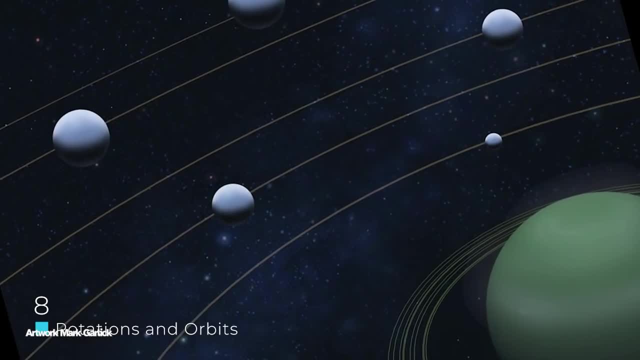 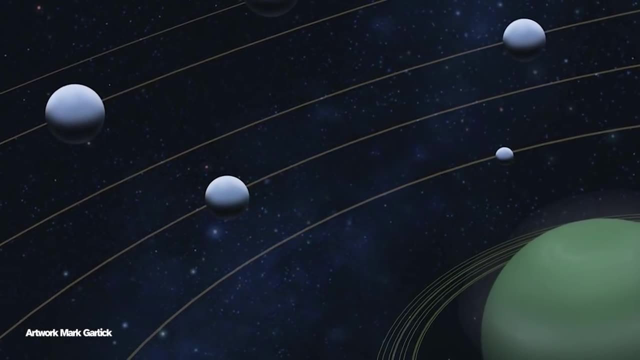 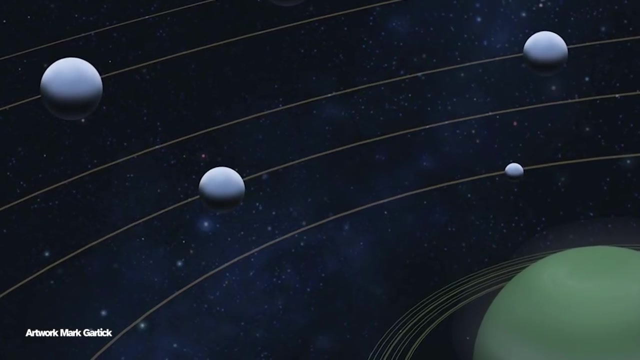 8. Rotations and orbits. Among Uranus' five major moons, Ariel is the second closest to the planet, orbiting at a distance of about 190,000 kilometers or over 118,000 miles. Its orbit has a small eccentricity and is inclined very little relative. to the equator of Uranus. Its orbital period is around 2.5 Earth days. coincident with its rotational period, This means that one side of the Moon always faces the planet, a condition known as tidal lock, which is a key thing in regards to temperature. more. 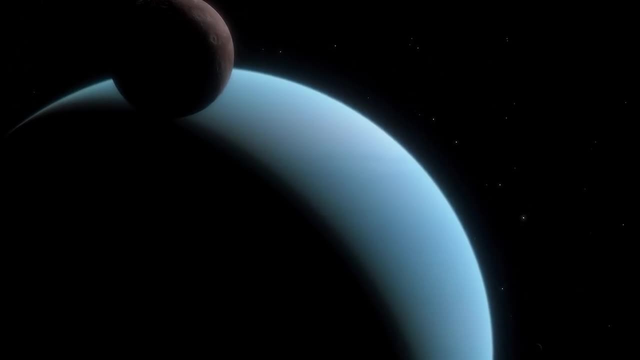 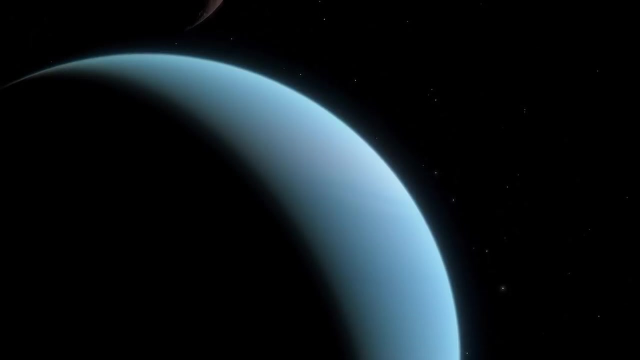 on that later. Ariel's orbit lies completely inside the Uranian magnetosphere. The trailing hemispheres, those facing away from their directions of orbit of airless satellites orbiting inside a magnetosphere like Ariel, are struck by magnetosphere plasma co-rotating. 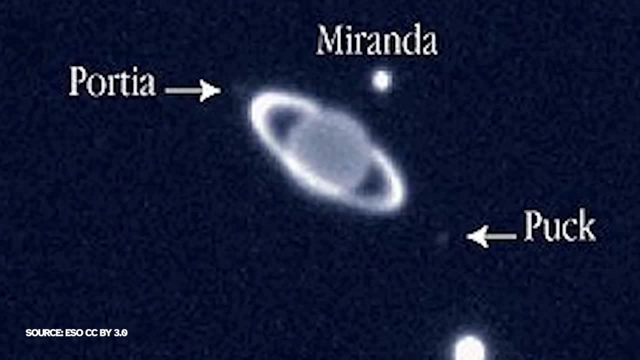 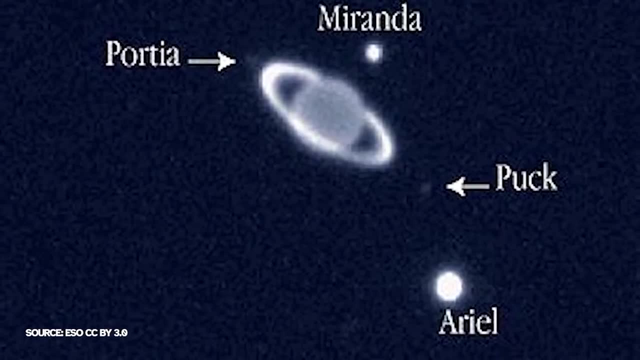 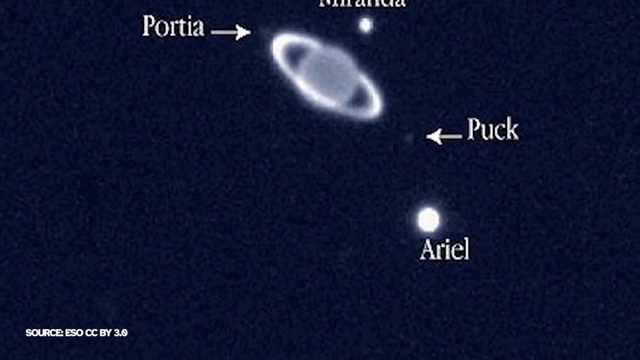 with the planet. This bombardment may lead to the darkening of the trailing hemispheres, observed for all Uranian moons except Oberon. Ariel also captures magnetospheric charged particles, producing a pronounced dip in energetic particle count near the Moon's orbit observed. 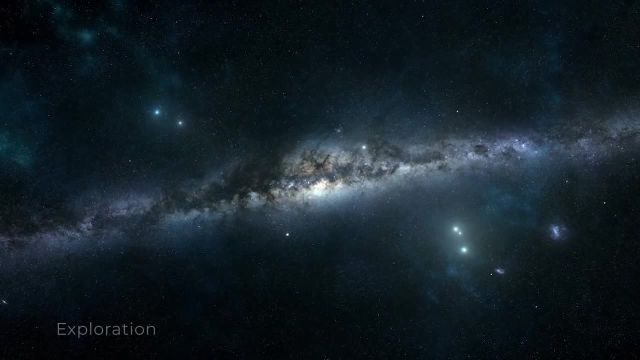 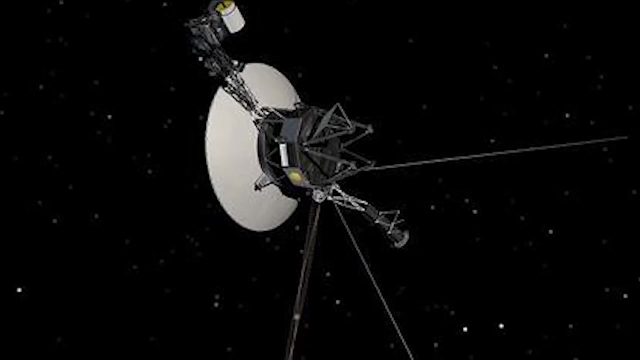 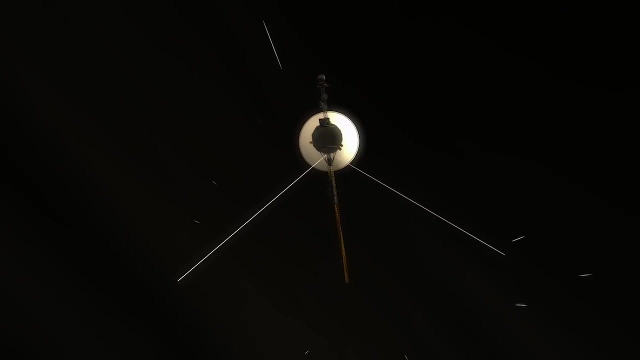 by Voyager 2.. 7. Observation and exploration. The only close-up images of Ariel were obtained by the Voyager 2 probe, one of the most important scientific tools in the history of the space program, which photographed the Moon during its flyby of Uranus in January 1986.. 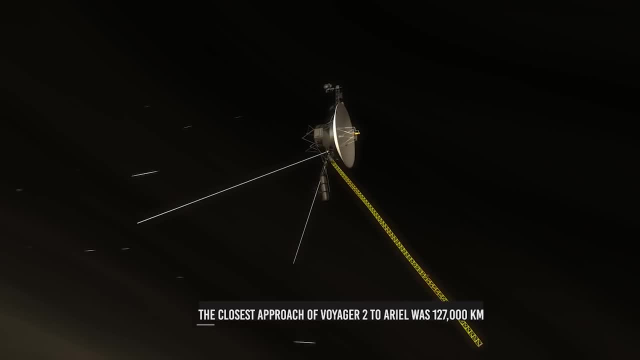 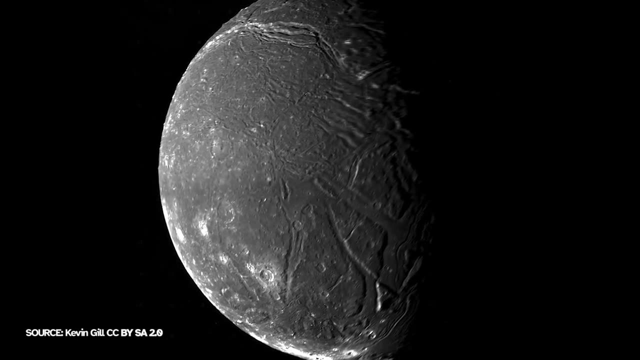 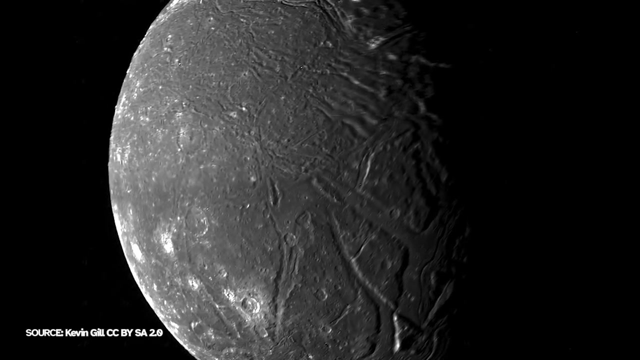 The closest approach of Voyager 2 to Ariel was 127,000 km, significantly less than the distance it covered by the Moon. The distance of Voyager 2 is 12 km and the distance it took to fly upon the Moon is around one meter, and the distance of Voyager 2 is 1. 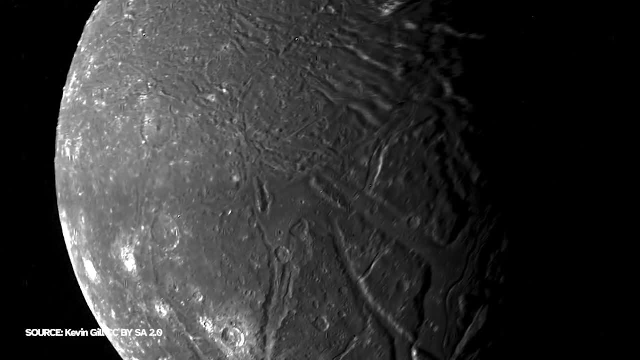 meter. The based mass of Voyager 2 is less than that of Uranus, and below that is the average mass of the moon, or 1 meter, which is 17.5, 8.. The moon's orbit is perfectly symmetrical, with atheletic-like formation which was 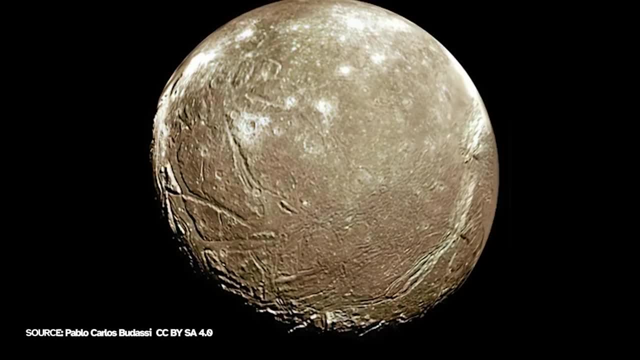 the basis for much of the Sun's orbit and the motion of the Moon. At the time of the flyby, the southern hemisphere of Ariel, like those of the other moons, was pointed towards the Sun. This means that the northern hemisphere of Ariel was automatically located in the 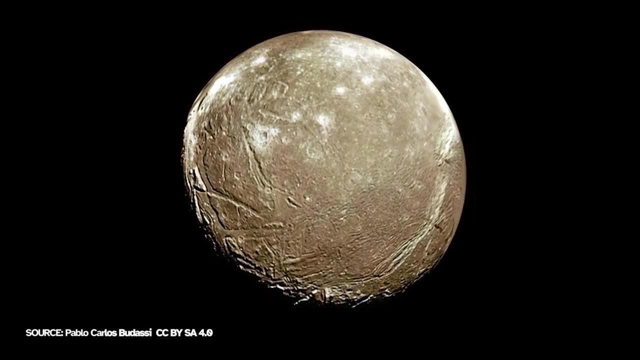 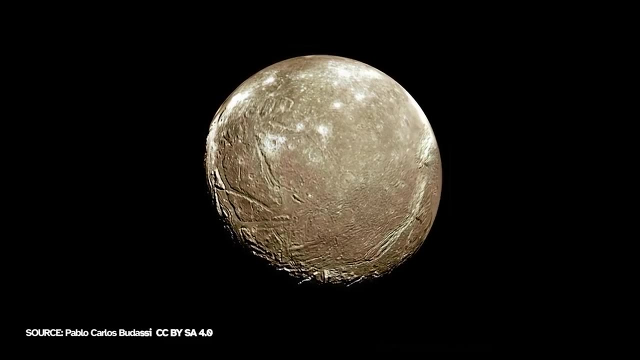 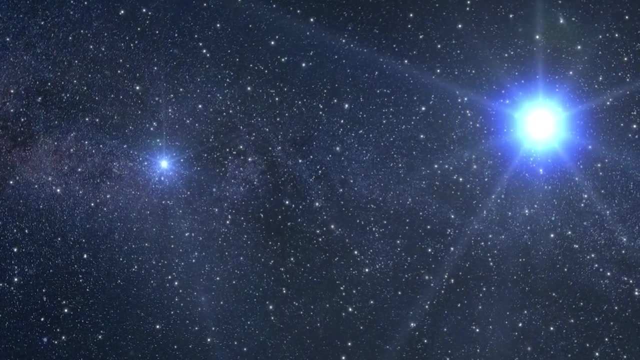 northern dark hemisphere could not be studied. No other spacecraft has ever visited the Uranian system. The possibility of sending the Cassini spacecraft to Uranus was evaluated during its mission extension planning phase. It would have taken about 20 years to get to the Uranian system after departing Saturn. 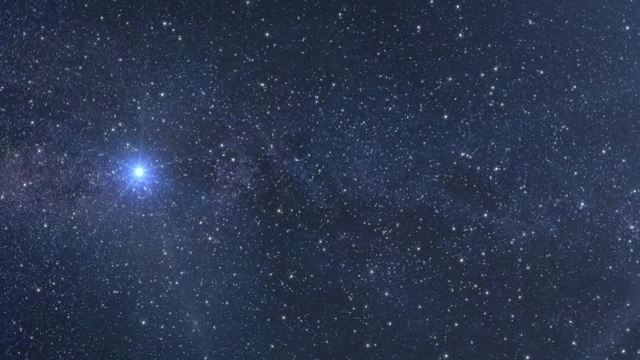 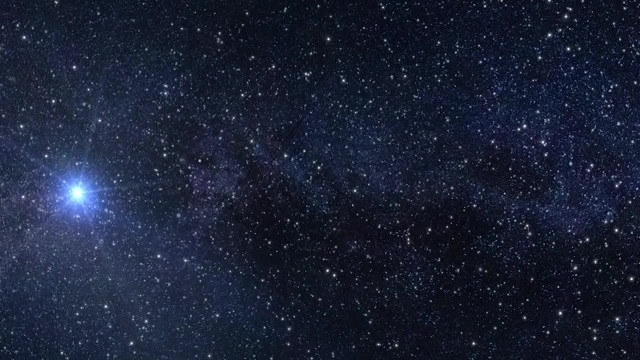 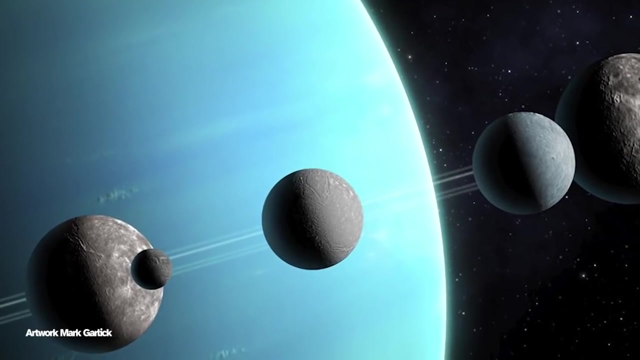 and these plans were scrapped in favor of remaining at Saturn and eventually destroying the spacecraft in Saturn's atmosphere. What this means on the whole is that there could be a chance to go and try to do a closer flyby for the Moon, should the opportunity arise, especially with the desire to further 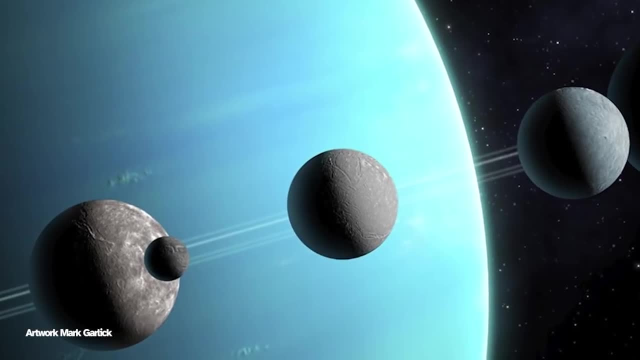 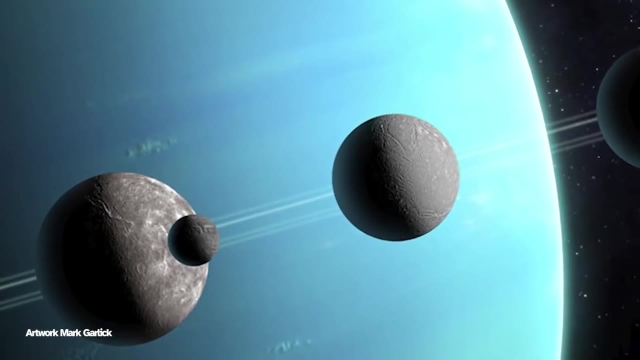 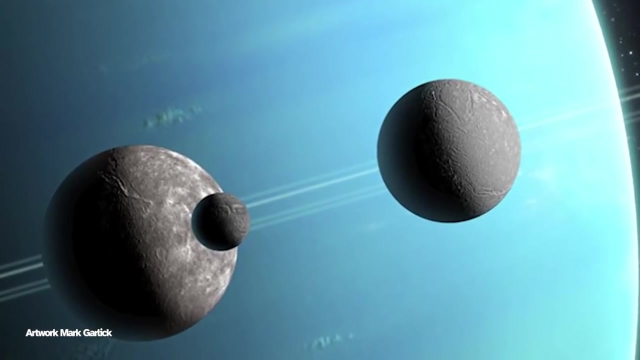 go and explore our solar system, growing with every year as we potentially get closer to sending a craft to Mars and other potentially viable spots in the solar system. If done correctly, it might not just go and help explore Ariel, but also explore the other moons of Uranus. 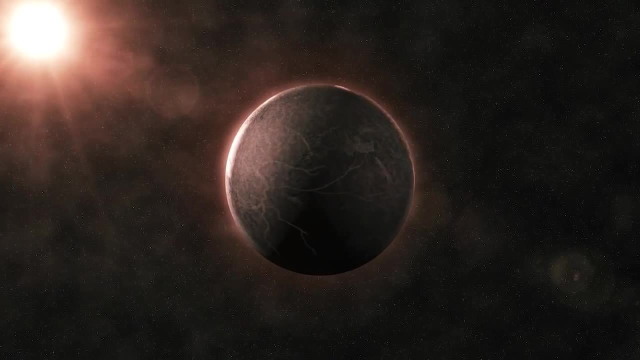 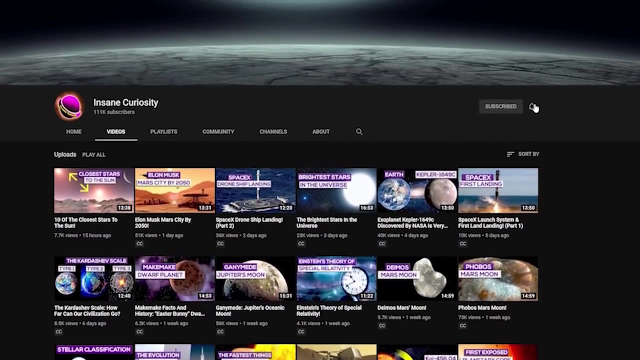 But whether this actually happens is up for debate. Before we continue, be sure to like or dislike the video and subscribe to the channel. that way we can continue to try and make the best videos possible for you, the viewers 6.. 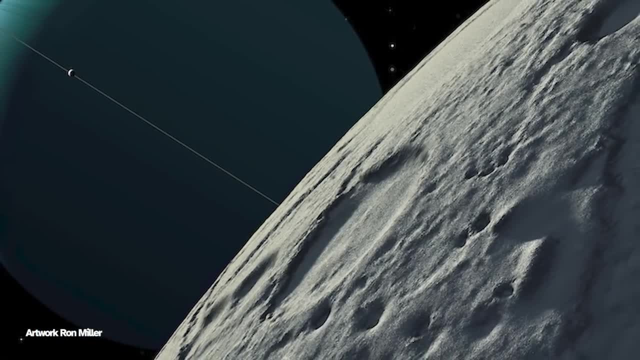 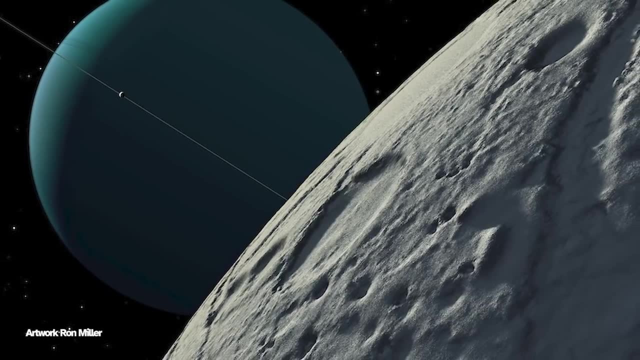 Atmosphere. Despite there being carbon dioxide on the moon of Ariel in some capacity, there is no detectable atmosphere or magnetosphere that we can find. While this may be, on the surface, sound like an okay thing, it's honestly not, Because when you want to look at the moon, you can't find it. 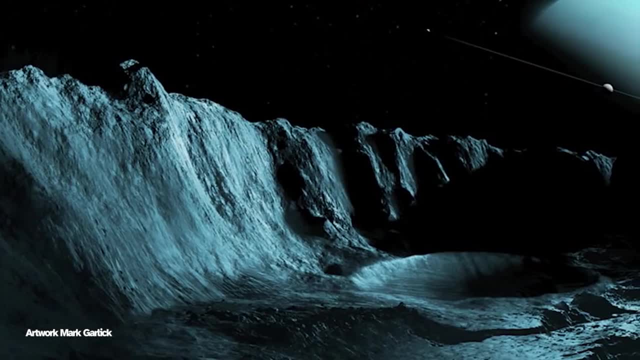 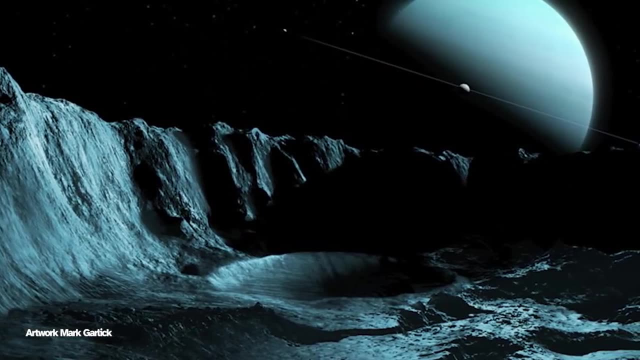 If you want to look for a place to live in the universe, an atmosphere is preferable for a variety of reasons. Without it and the magnetic field, it means that not only will anything on the surface be open to getting hit by various cosmic rays, it makes it all the more likely that asteroids 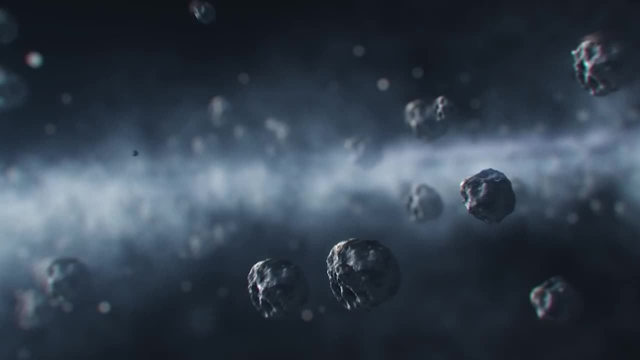 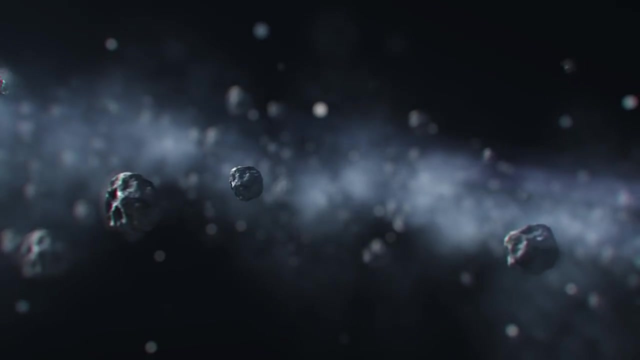 and meteors will bombard the place, Which, if you recall, is something we know happens on Ariel, especially with the smaller space rocks. Now, to be clear, this doesn't make it the most uninhabitable place ever, but it is a. 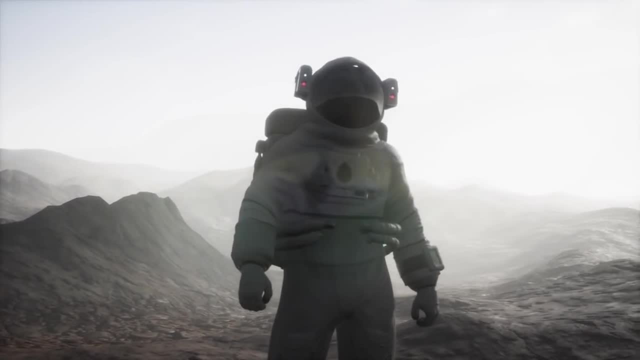 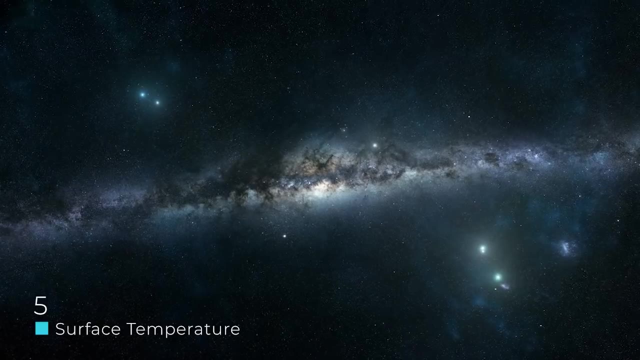 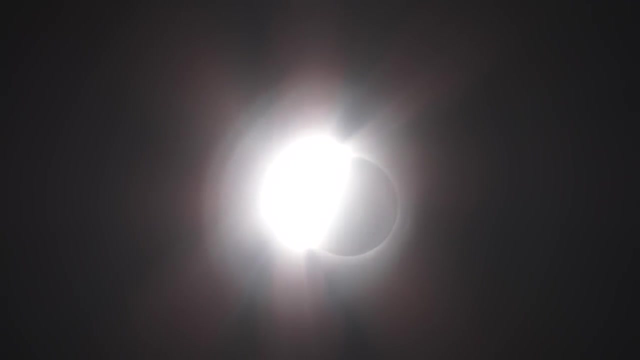 major deterrent in terms of exploration And wanting to go there for one reason or another, to colonize. 5. Surface temperature Measurements have shown that Ariel's surface temperature rises and falls quickly with the coming and going of sunlight, without a thermal inertial lag. 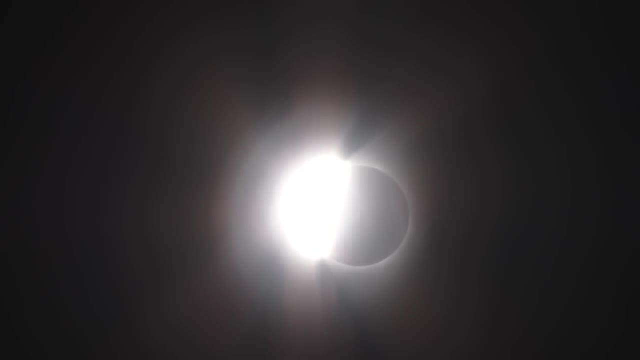 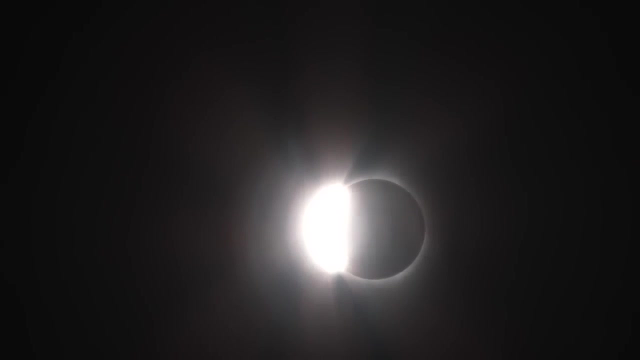 That supports the picture of a porous surface, which would tend to insulate the moon and keep the subsurface from heating up. This texture could be the result of eons of micrometeorite strikes tilling the soil. 7. Temperature difference In earlier time Ariel appears to have undergone. 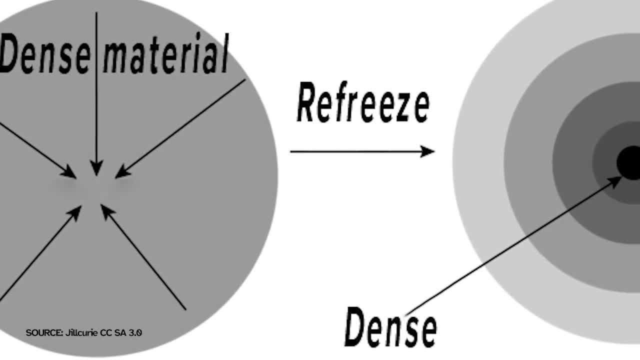 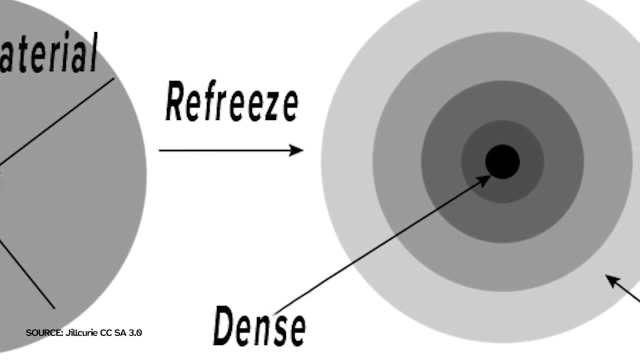 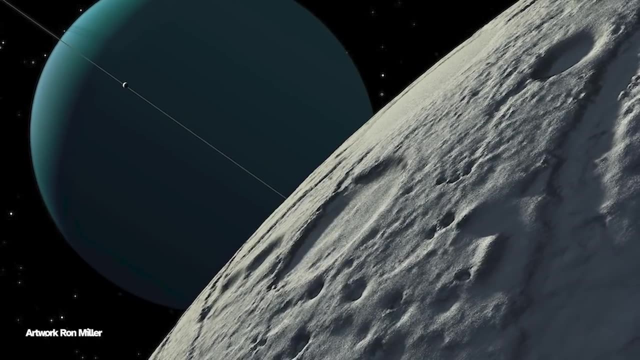 enough heating to allow differentiation, a separation in which heavier materials sink towards the core and lighter material floats at or near the surface. Models indicate that tidal interactions with Uranus may provide an important source of heat, But whether that heat is enough to do certain things, including live on the surface by channeling. 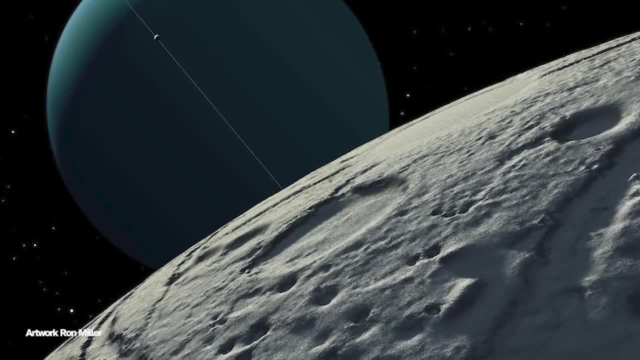 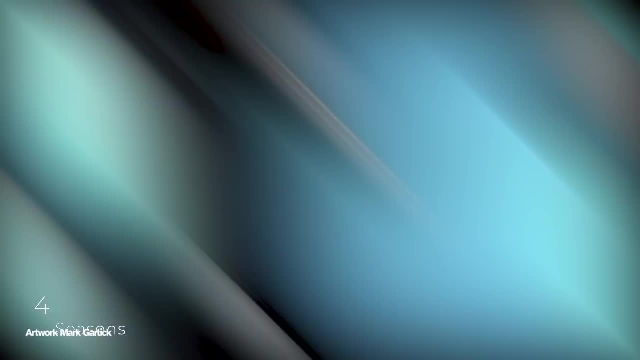 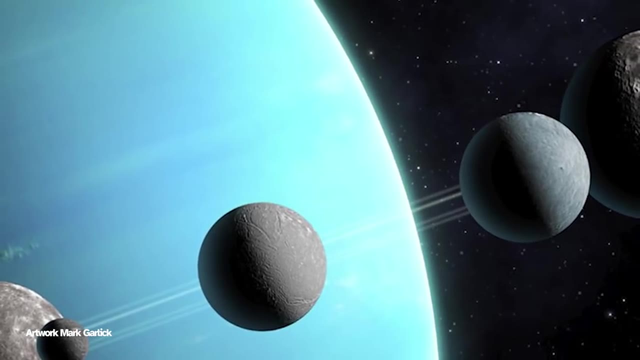 that heat is up for debate, but given how the moon is in tidal lock and that the temperatures rise and fall, It's unlikely 4. Seasons, Because Ariel, like Uranus, orbits the sun almost on its side relative to its rotation, its northern and southern hemispheres face